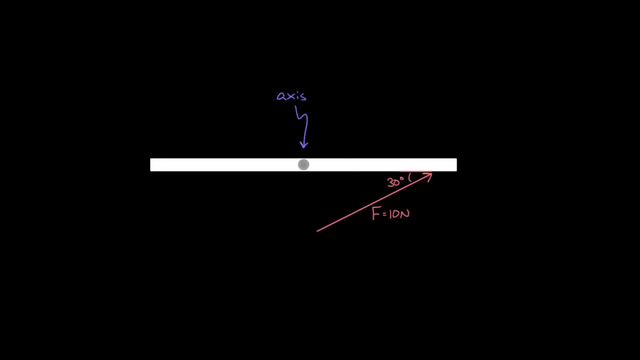 because if a force is gonna exert a torque, it has to be applied at some point besides the axis. In other words, if you go try to push open this revolving glass door at the very center, nothing's gonna happen because it's not gonna rotate. 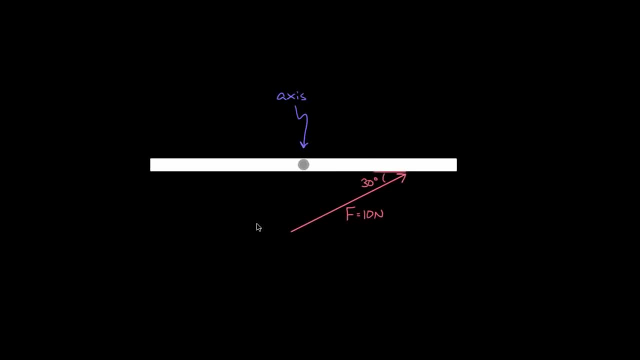 But the farther out you apply this force, the more torque you will get for the amount of force that you're exerting. So a force out here would apply much more torque than a force right here. That's why the doorknobs are near the edge of the door. 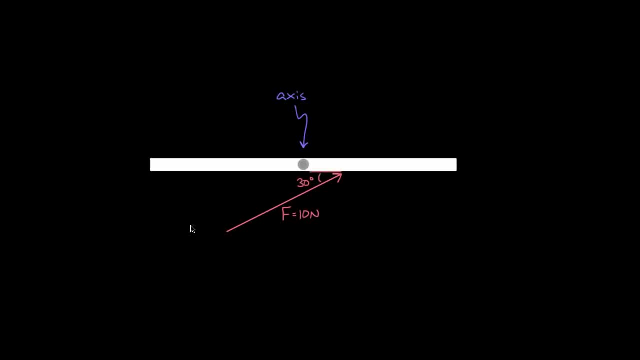 It'd be really hard to open a door right near the hinge. If you haven't tried it, try it out. It's really hard. Now that we've identified the axis, we could figure out how much torque we're exerting. Now the first thing I might try to figure out the torque here. 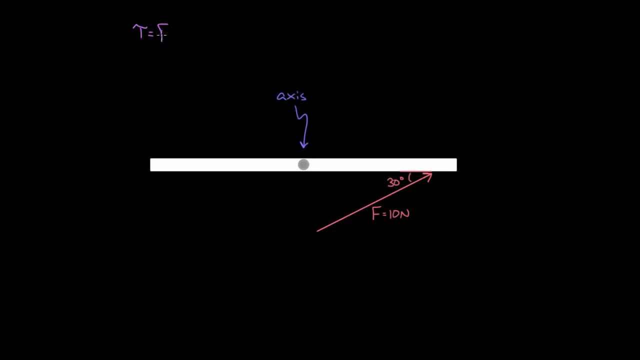 is- I'd just say all right- torque. I know what torque is. Torque is F times D or F times R. you could call it an R, But what's important to know is that this R represents the vector that points from the axis. 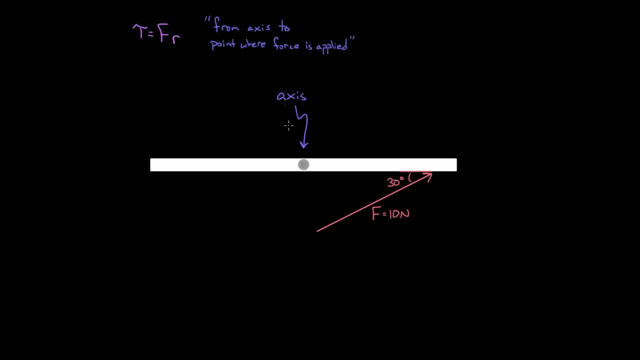 to the point where the force was applied. So in this case that would represent- from this axis right here to the point where the force was applied- would be this: This would be R. Note that R is not the entire radius, necessarily, and it's not the entire length of the object. 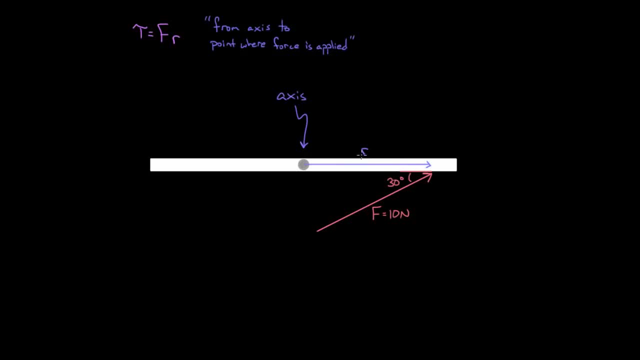 always from the axis to the point where the force is applied. And technically this R is a vector- You can think of it as a position vector- but regardless, it points from the axis to the point where the force is applied. It doesn't point the other way. 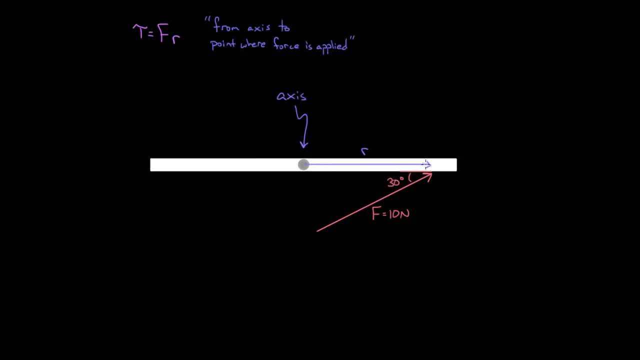 The direction is not toward the axis. The direction is always away from the axis to that point Where the force happens to be applied to the object. So let's give this a number. Let's say this happened to be two meters from this axis. 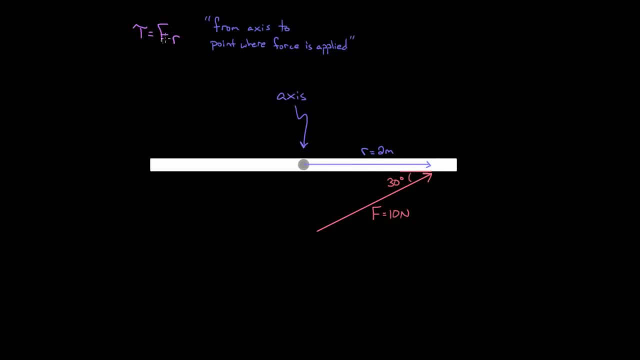 to the point where this 10 newtons was applied. Now we can solve for this torque, but you have to be careful. A mistake I might have made is to say just well, the force was 10 newtons. the R here is two meters. 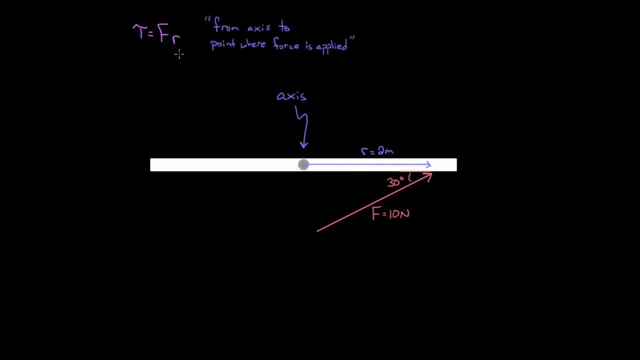 so my torque should just be 20, right, Two times 10?. But that's not right, because this force is not representing the total force necessarily. If you just write this formula for torque like this, what you really mean is that this force is the perpendicular. 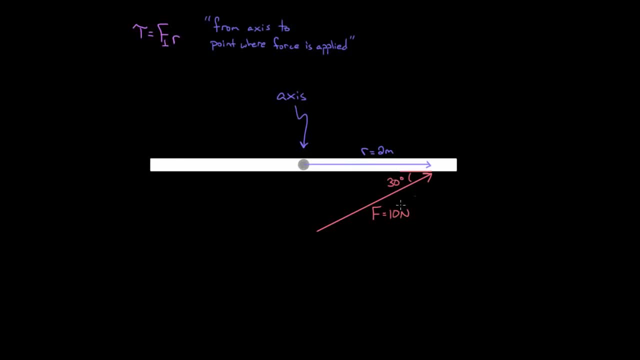 perpendicular force to this R, So only the perpendicular component of this force is gonna exert a torque on the door. The component parallel to the R doesn't exert any torque and that should make sense. So if I draw this out, let me draw the components. 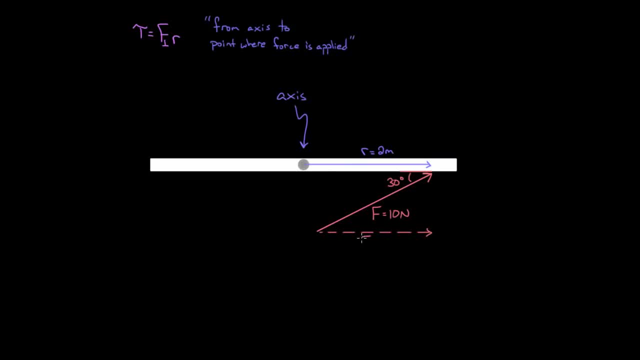 If I break this 10 newtons up into a component that goes this way, I'll call that F parallel, because that force is parallel to R. It runs the same direction as R does, And I'll break it up into this component as well. 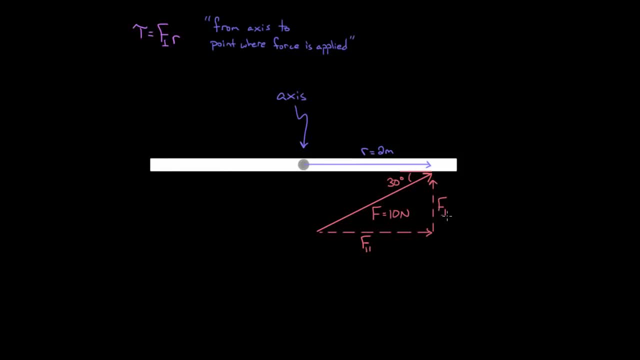 this perpendicular component, and I'll call that F perpendicular. so this component is perpendicular to this R vector. Only this perpendicular component is gonna exert a torque, and that should make sense. Torque is a force that causes something to start rotating or to change its rotation. 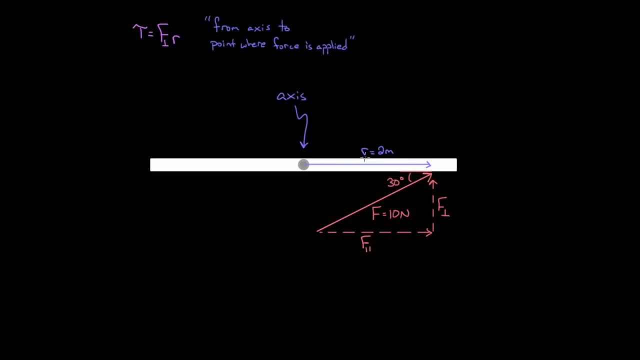 So the only component of this force, of this 10 newtons that is gonna cause this door to rotate is this perpendicular component. This is the way you push on a door to make it rotate. You don't pull the axis this way. 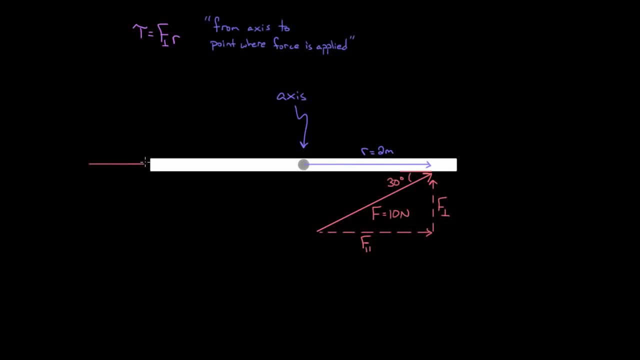 If I came up and tried to open this revolving glass door by pushing that way, that's crazy, because that's not gonna cause the door to rotate. Similarly, trying to pull the door that way is not gonna cause this door to rotate. You need to exert a force perpendicular to this R vector. 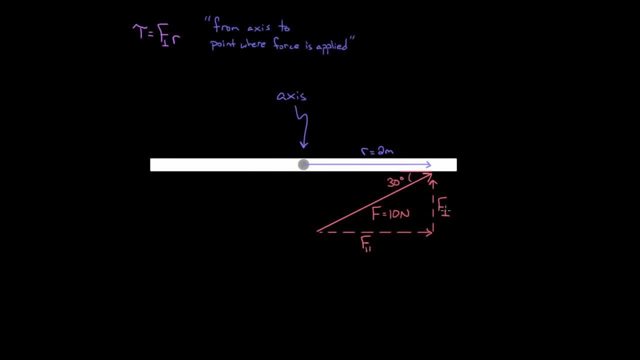 in order to get the door to rotate. In other words, only perpendicular components of the force, that is, perpendicular to the R, are going to exert a torque. So it's only this component of the 10 newtons that's going to contribute toward the torque. 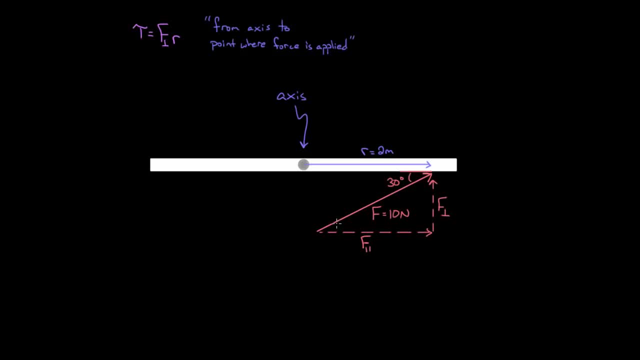 And we can find that If this was 30 degrees, this is an alternate interior angle. That means this is also 30 degrees, So these angles are identical. based on geometry, That means this component that's perpendicular. I can write as well. let's see. 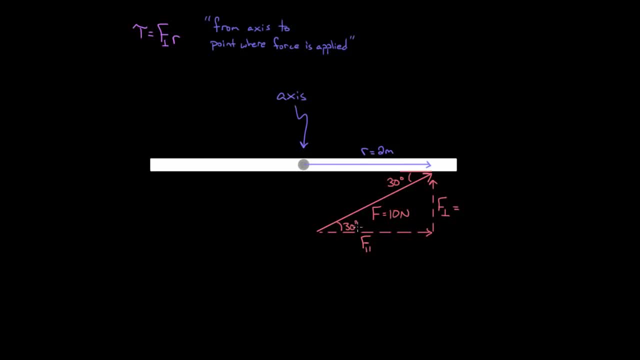 it's the opposite side. That side is opposite of this 30 degrees. So I can say that it's gonna be 10 newtons. The hypotenuse would be 10 newtons times sine of 30. And 10 newtons times sine of 30 degrees is five newtons. 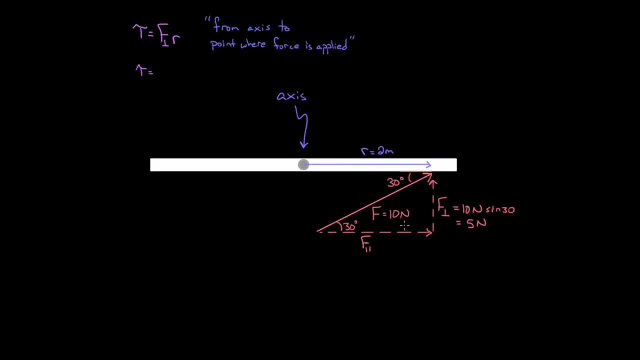 So, finally, I can say that the torque exerted on this door by this force of 10 newtons at 30 degrees, by this force of 10 newtons at 30 degrees, would be the perpendicular component, which is five newtons. 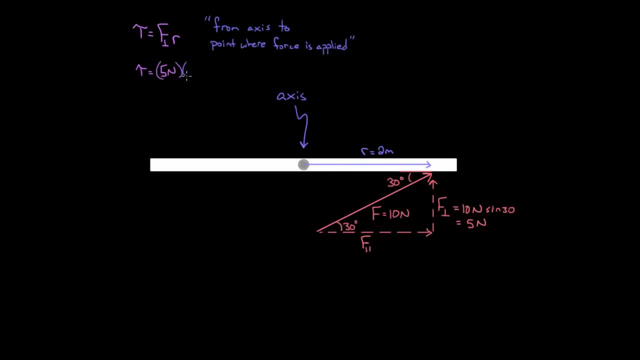 times how far that force was applied from the axis, And that was two meters. And I get that the torque here is gonna be 10 newton meters. So at this point I wouldn't blame you if you weren't like. see, this is why I hate torque. 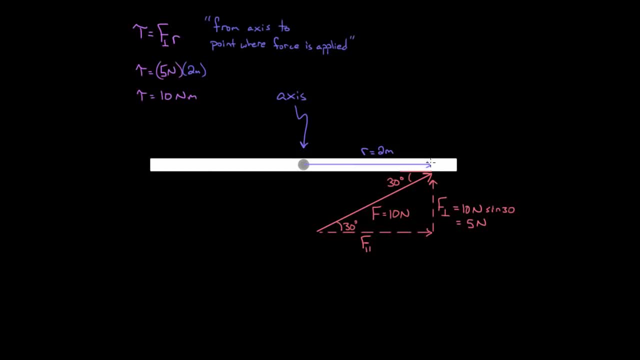 I've got to remember that this two meters is from the axis to the point where the force is applied. I've got to remember that I'm only supposed to take the perpendicular component And I'm supposed to remember that perpendicular means perpendicular to this R vector. 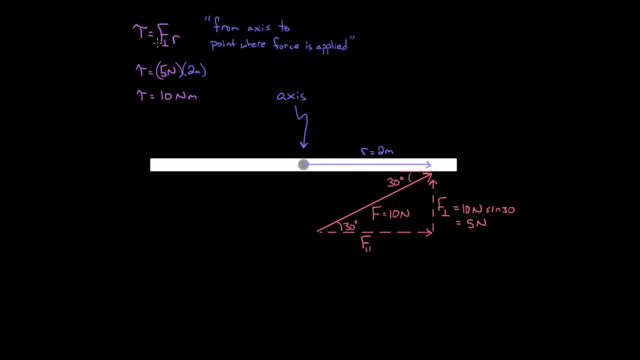 You might wonder: is there an easier way to do this? Is there a formula that makes it so I don't have to carry so much cognitive load when I'm trying to solve these problems? And there is, since this force component is always the component that's perpendicular to the R. 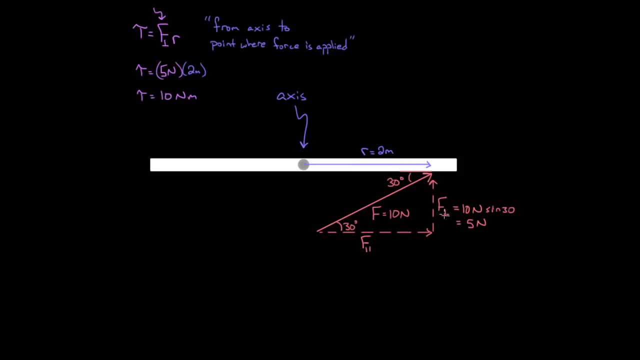 we can take that into account when writing down the formula. In other words, the way you find that perpendicular component is by taking the magnitude of the total force, the 10 newtons, and you multiply by sine of the angle between the R vector and the F vector. 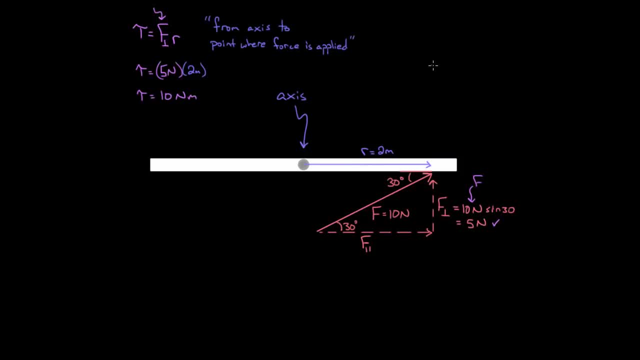 That's what we did to get this five newtons. So why not just write down this formula explicitly in terms of the total force times sine theta, that's gonna be the perpendicular component- and then multiply by R. So what this represents is this here: 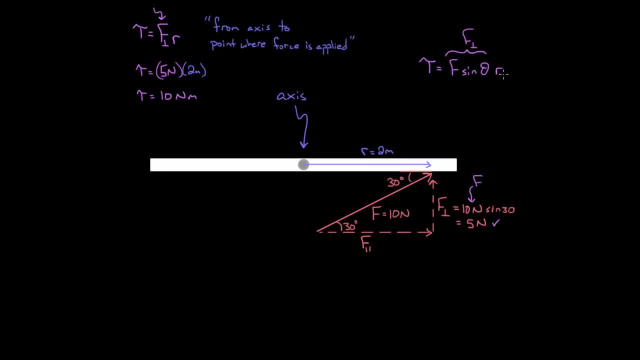 this F sine theta is F perpendicular, And then you multiply by R, just like we always do Now in most textbooks you'll see it written like this: They like putting the sine theta at the end Looks a little cleaner. So if we do F times R, times sine theta. 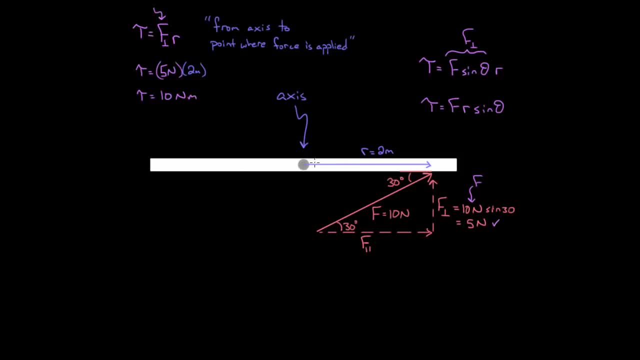 now we can just plug in the entire 10 newtons in for the force, the entire two meters in for the R, and this theta would be the angle between the force and the R vector. but that's crucial. You've gotta remember if you're gonna use this formula. 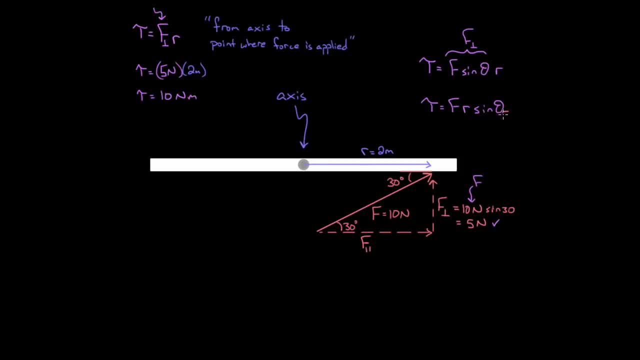 instead of this formula. you've gotta remember that this angle here is always the angle between the force vector and the R vector, which is the vector from the axis to the point where the force is applied, which in this case was 30 degrees. 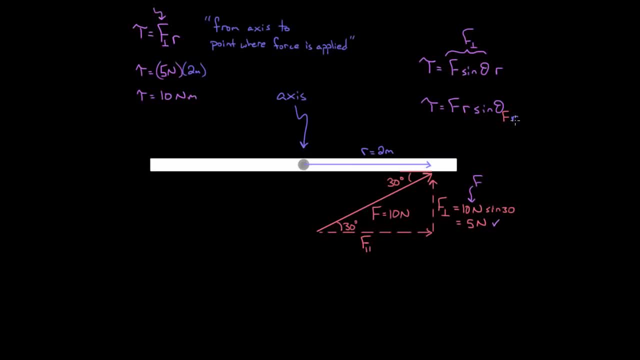 So sometimes it's not obvious. How do you figure out the angle between F and R? Well, first you identify the direction of F and the direction of R. The safest way to figure it out would be to imagine taking this F vector and just moving it. 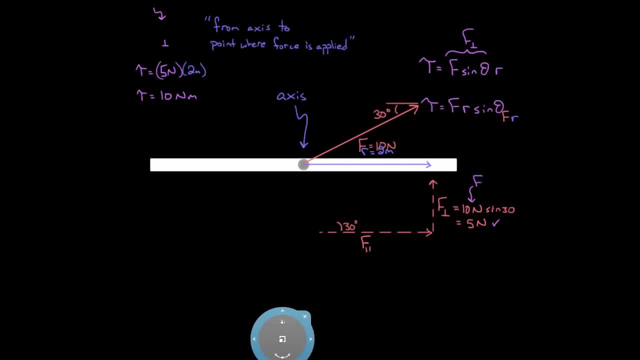 so its tail is at the tail of the R vector. and then you'd wanna figure out, okay, how much angle is there between this F and this R? Well, alternate interior angles. again, that makes 30.. So that is the angle. 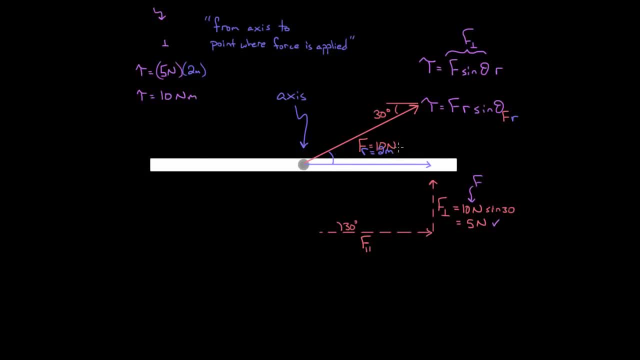 The angle between the F vector and the R vector is the angle we're looking for when we're solving for the torque exerted by a certain force, So let's use this formula. Let me take this formula. We're gonna use this to solve another example. 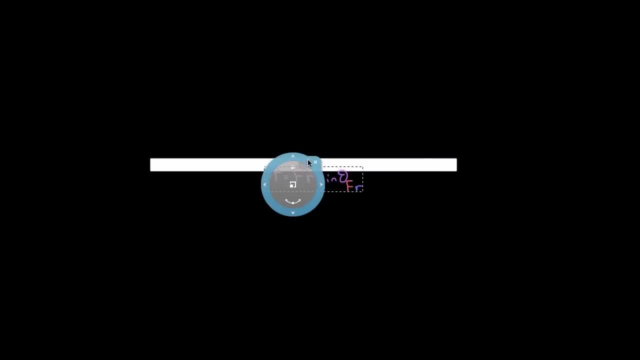 because the only way to get good at this and to not fear it is to practice a few. Let's take our new formula: Torque is F? R sine theta. Let's say there was a force applied right here, and let's say you were given these distances here. 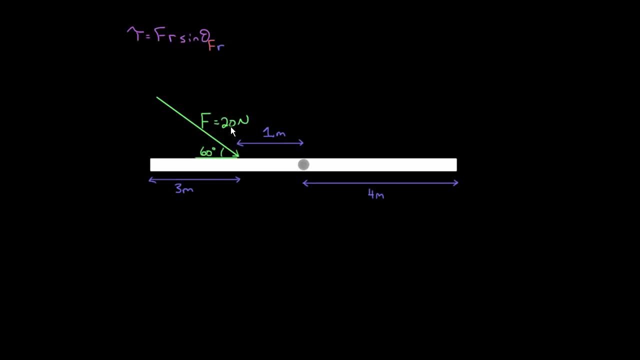 and we wanna figure out how much torque does this force of 20 newtons apply if it's at this angle of 60 degrees? So we'll use our formula. We're gonna use this. F is the entire F. Now we don't have to break the F into components. 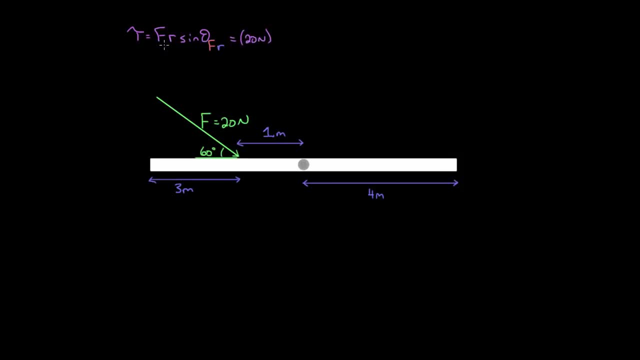 We can just say that it's the entire 20 newtons of force of the force times R. but we got all these. We got three different Rs here. Which one do we use? Remember, R is defined to be from the axis. 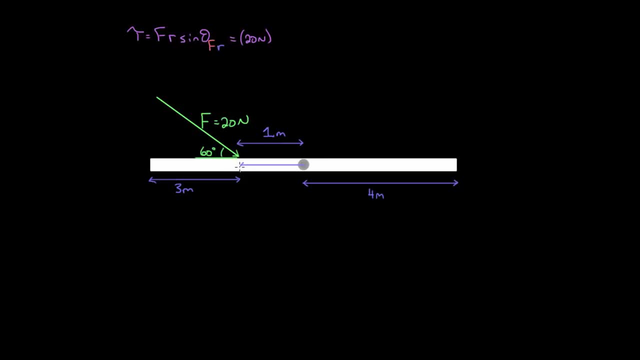 which again is gonna be in the middle to the point where the force was applied. That's this way. so the magnitude of R is one, It's not three, it's not four. If you're given multiple numbers, you have to be careful. 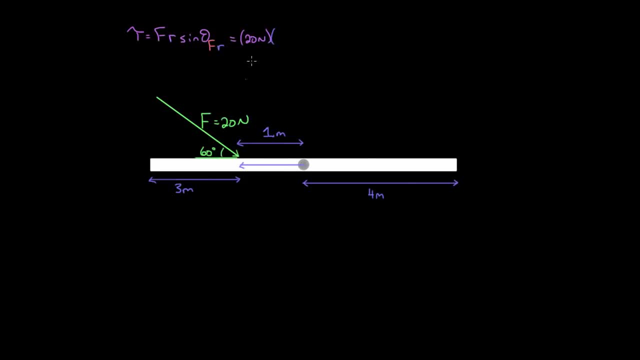 You have to select that vector that goes from the axis to the point where the force is applied. So this is the magnitude of that vector, which is one meter, And then it's gonna be sine of the angle between the force vector and the R vector. 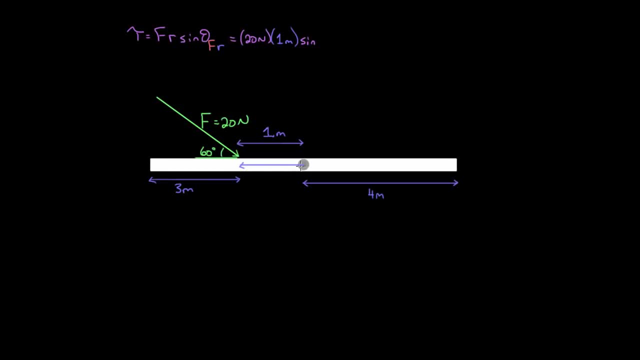 So think about it. force goes this way: down and right, R goes to the left. The true angle between R and F would be: we'd have to imagine moving F so that they're tail to tail, And we could say that F is gonna point down and right. 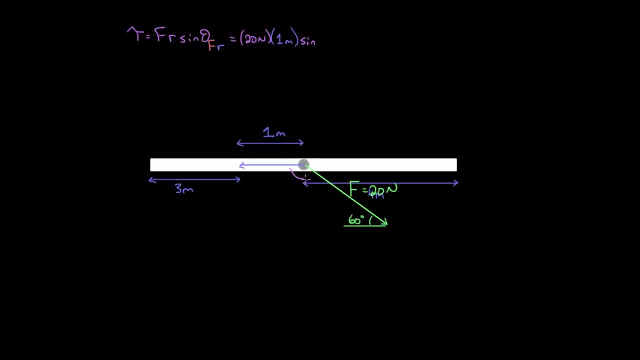 R goes to the left, The angle between them would be this much angle. Now we can find that in a variety of ways. One thing we could do is imagine making a right triangle here, If that's 60 degrees and this is 90,. 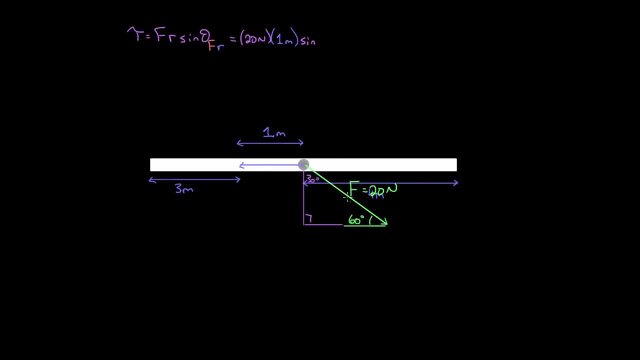 then this has to be 30 degrees, since the interior angles of a triangle have to add up to 180.. And if that's 30 and this is 90, then that angle has to be 120. So we can stick 120 degrees up here. 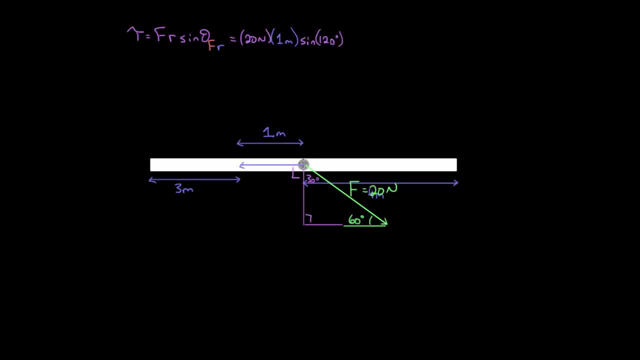 as the actual angle between the force vector and the R vector. Now, if you missed that, the reason we're saying 120 is because 90 plus 30 is 120. So if the angle between R and F is 90 degrees plus 30 degrees, then it's gonna be 120 degrees. 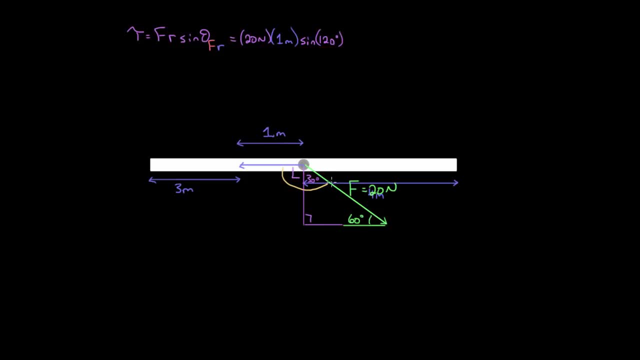 That's why we're putting 120 up here as the angle between R and F. But you might be concerned, You might be like that was a lot of work. I don't wanna have to do that. I just wanna take my F vector. 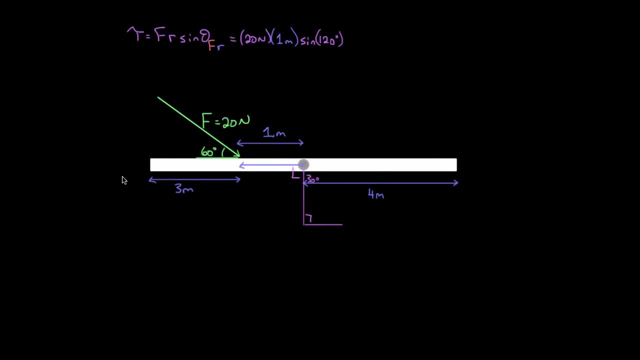 and determine what the angle is between F and R. Do I really have to imagine moving it? And you don't? so it's not that hard. Yes, technically, tail to tail is the way to determine the angle between two vectors, but head to head gives you the same angle. 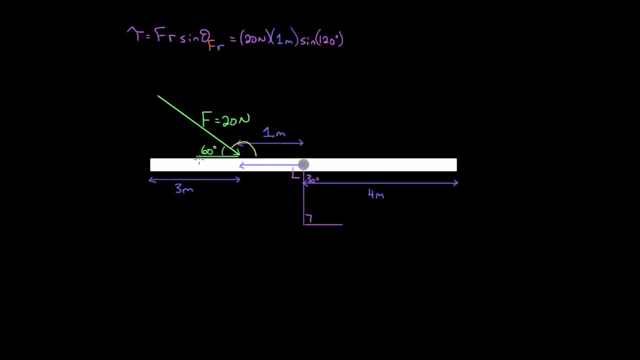 So I could've just looked at this angle here. I knew that this was 60, and I knew 180 minus 60 gives me 120.. So that's another way to figure out the angle you put into here. So, in other words, you do not have to imagine. 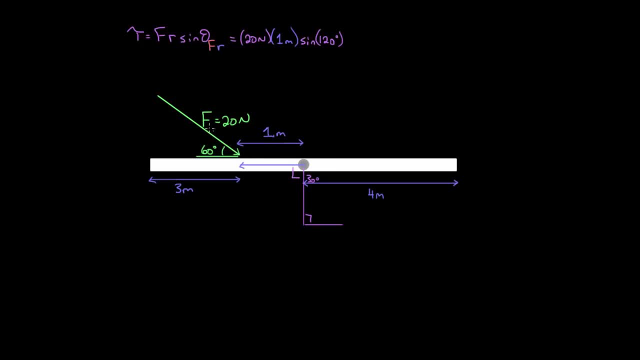 moving this vector tail to tail If the vectors are butting heads. if you have your F vector and your R vector butting heads, just find the angle between the F vector and the R vector. that way It'll still give you the same angle, which is 120 degrees. 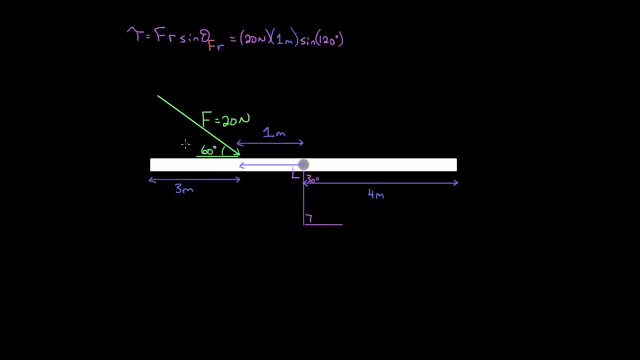 Now you might wonder: what if I totally screw up? What if, instead of putting in 120, I just throw in the 60?? I mean, that was the angle that was given. What would happen then? Turns out, you'd still get the right answer. 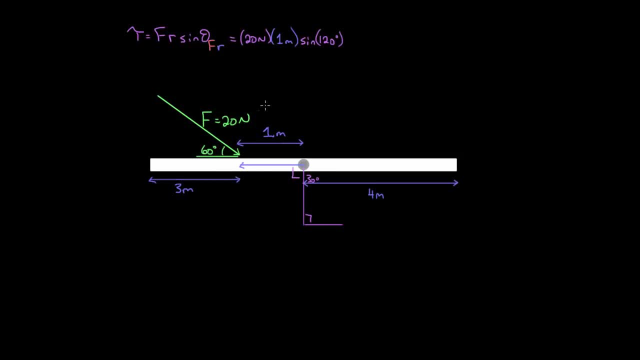 The torque formula is kind in this sense, Because even if I put in 60, sine of 60 is the same as sine of 120. That's not a coincidence here. It's because this angle here, this 120 between F and R, 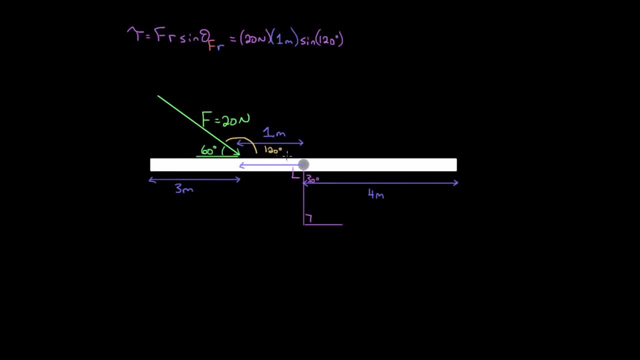 is supplementary to this 60 degrees. Think about it: this whole angle from this point all the way to there is 180.. If this is 120, this 60 degrees would have to be the supplementary angle, because these have to add up to 180.. 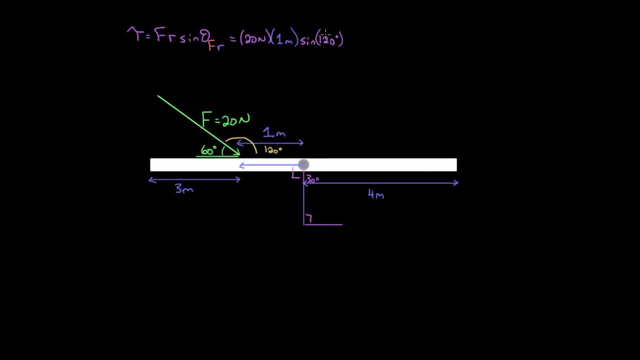 And the sine of supplementary angles gives you the same answer. So if I plug in 60 degrees up here, it would still work. So long story short, even though we define the angle between vectors as the angle between them when they're tail to tail, you put them head to head. 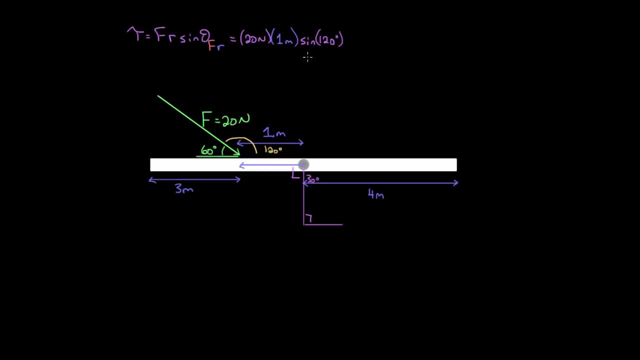 that still gives you the same angle as tail to tail, And since we're taking sine of that angle, we can use either of these supplementary angles to get the same answer. So just stick your F vector next to your R vector. find either of these angles. 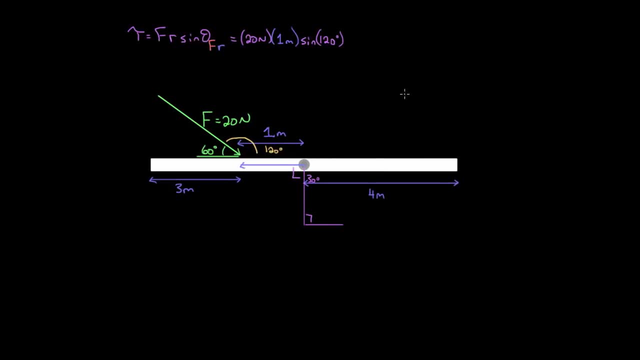 You can use that in this torque formula and you'll get the right answer. So, recapping, you can find the torque from a force by taking the perpendicular component of that force and multiplying by the magnitude of the R vector, where this R vector is the vector that points. 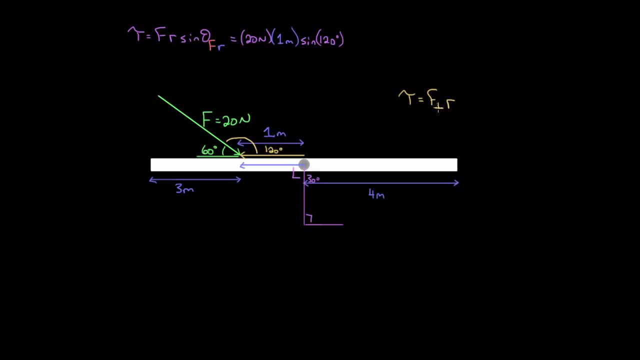 from the axis to the point where the force is applied, And by perpendicular we mean perpendicular to the R vector. Or you could use this formula, where F would represent the entire magnitude of the force, R would be the magnitude of the R vector. 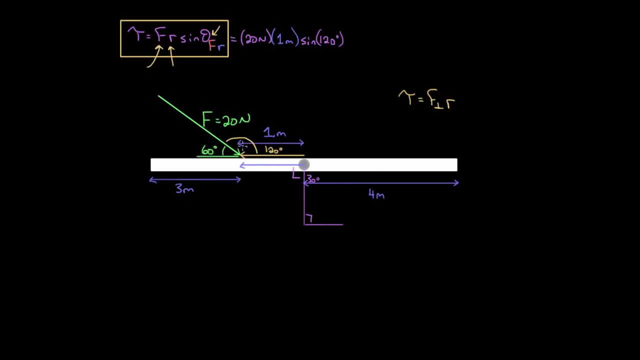 and the theta in here represents the angle between the force and the R vector. when they're head to head, when they're tail to tail, or because, sine of supplementary angles are equal, you could also take the supplementary angle to that angle between F and R.